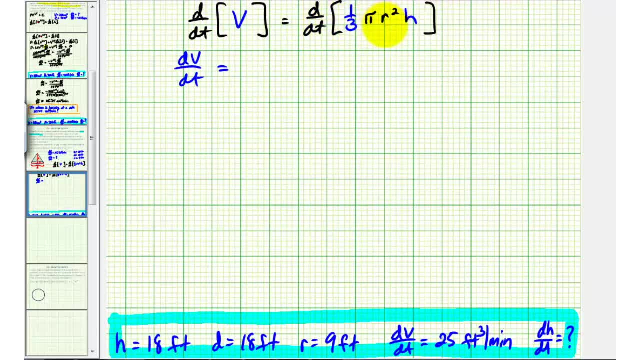 equals on the right side, the derivative of one-third pi R squared H with respect to T would be one-third pi times the derivative of R squared times H. So again we're going to apply the product rule. So we'll have the first function, R squared times the derivative of the second function. 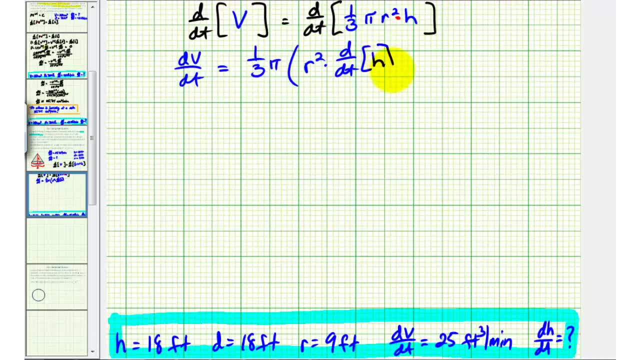 with respect to T, plus the second function, which is H, times the derivative of the first function with respect to T, which is R squared. Now let's go ahead and find these two derivatives and then we'll solve for DH DT. 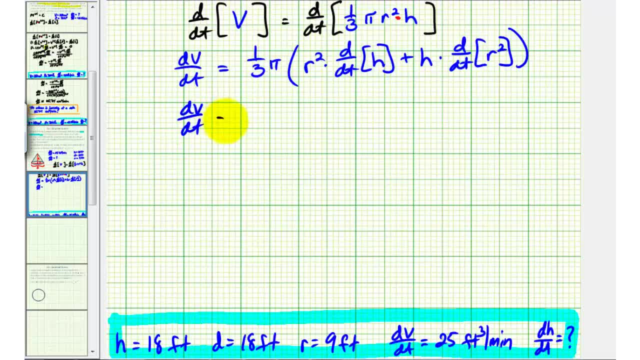 So we have: DV. DT equals one-third pi Times R squared times the derivative of H. with respect to T would just be 1 times DH DT or DH DT. Remember this is what we're trying to solve for, plus H times the derivative. 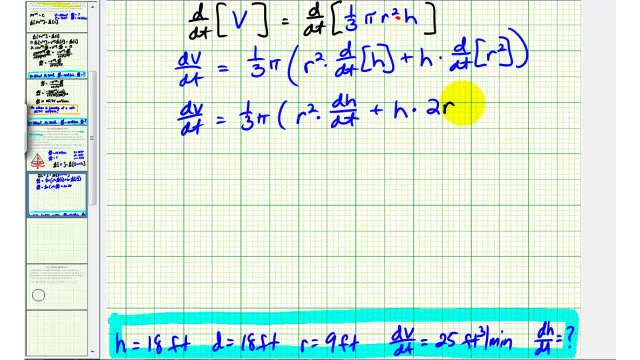 of R squared with respect to T would be 2 times R to the first, or just 2R times a factor of DR DT. Now let's start performing substitution so that we can find DH DT. We know DV DT is equal to 25 cubic feet per minute. 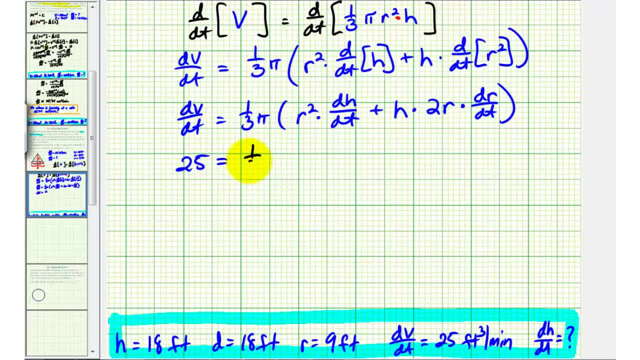 So we have 25 equals one-third pi times R squared. Well, we know R is 9, so we'd have 9 squared times DH DT, which we're trying to solve for, Plus H, which we know is 18 feet times 2, times R, we know is 9, times DR DT. 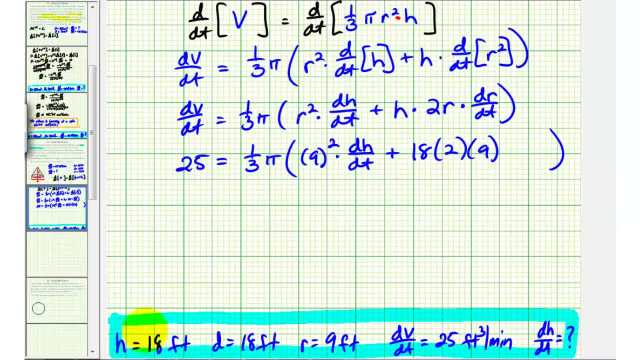 We need to think about DR DT for a moment. Remember, we were told the height and diameter were always equal to each other, and we know that the radius is always half the diameter and therefore the radius is also always half the height. So the radius is always half the height. 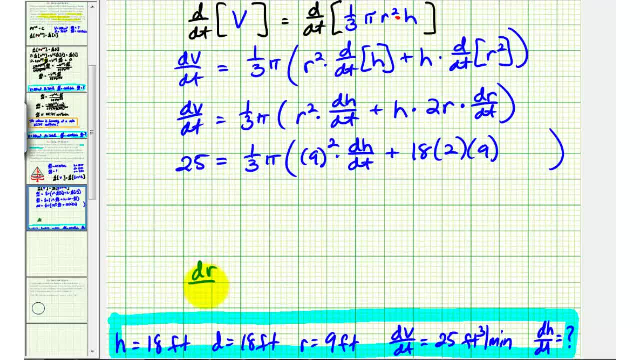 That means DR DT, or the change in the radius with respect to time, would always have to be half DH DT, or half the change in the height with respect to time, So we can substitute one-half DH DT for DR DT. The reason this is so helpful is now we only have one unknown in our equation, which is DH DT. 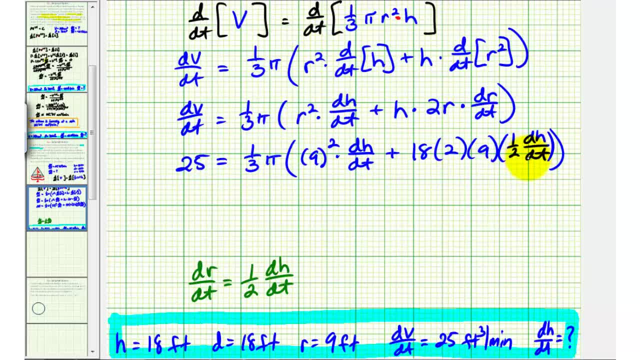 So now we'll solve this for DH DT in order to determine the rate of change of the height with respect to time. So we'll have 25 equals 1 3rd pi times the quantity. This will be 81 dh dt. 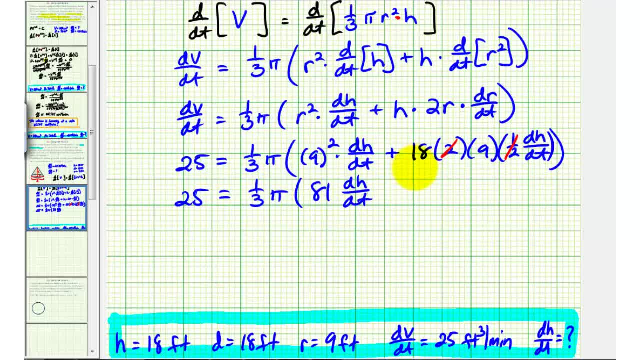 Notice here: the two and the 1 1⁄2 simplifies to one. 18 times nine is equal to 162.. So we have plus 162 dh dt. Let's go ahead and multiply both sides of the equation by three. 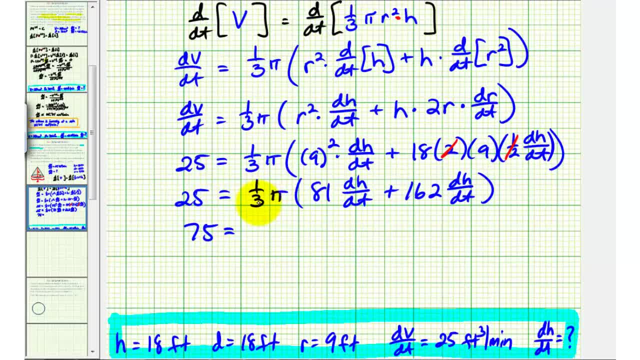 So three times 25 is 75.. Three times 1, 3rd is just one. So we have pi times the quantity 81 plus 162 is 243.. So we have 243 dh dt. So to solve for dh dt we'll divide both sides by 243 pi. 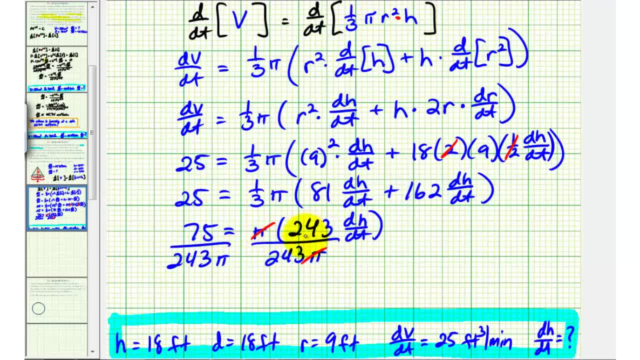 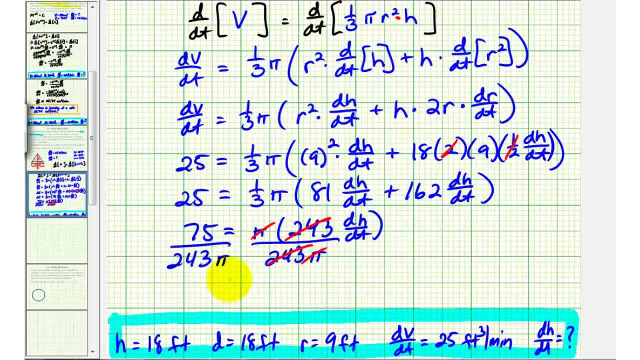 So pi over pi simplifies to one, 243 over 243 simplifies to one. Notice how we now have this all for dh dt. dh dt is approximately equal to 0.0982.. Again, this is the change in the height with respect to time. 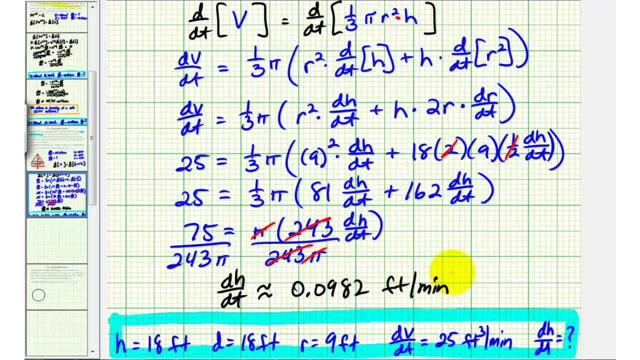 So this would be feet per minute, Which means, under these conditions, the height is increasing at a rate of approximately 0.0982 feet per minute. Keep in mind, if any of these conditions were different, that would affect the value of dh dt. 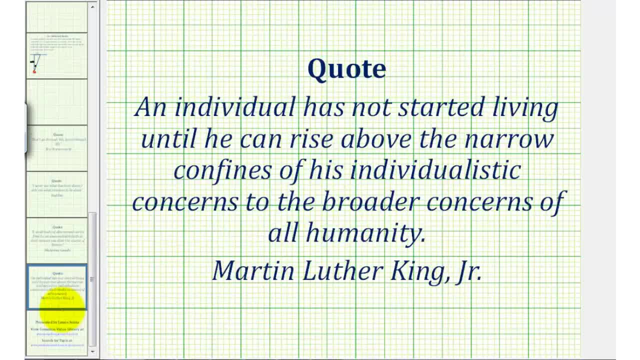 I hope you found this explanation helpful. Thank you for watching.